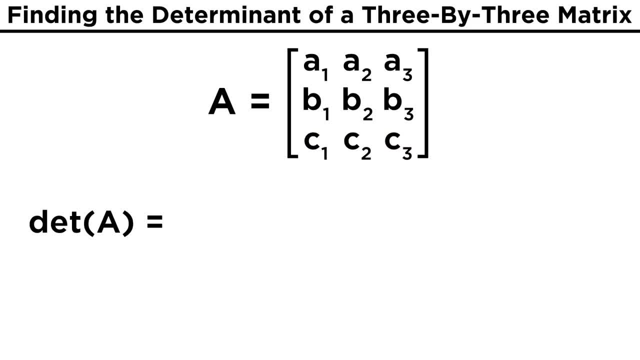 and C one, C two, C three. Finding the determinant of this will already be much more complicated than for a two by two matrix, because its determinant must be the determinant of a two by two matrix. So let's look at a two by two matrix. 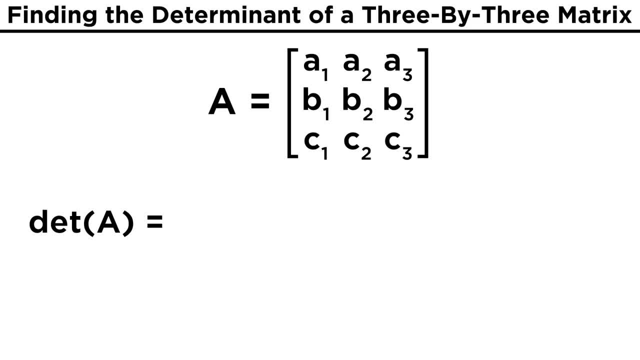 Let's look at a two by two matrix. It must be broken down into a series of second order determinants. We will take A one and multiply it by the determinant of a new two by two matrix comprised of B two, B three, C two and C three. 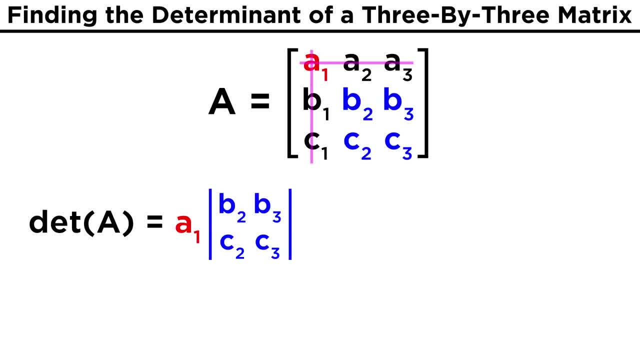 So it's like we ignored the row and column that A one is a part of and kept the rest for a new matrix. From this we subtract A two times the determinant of another two by two matrix, This time ignoring the row and column that A two is a part of, leaving us with B one. 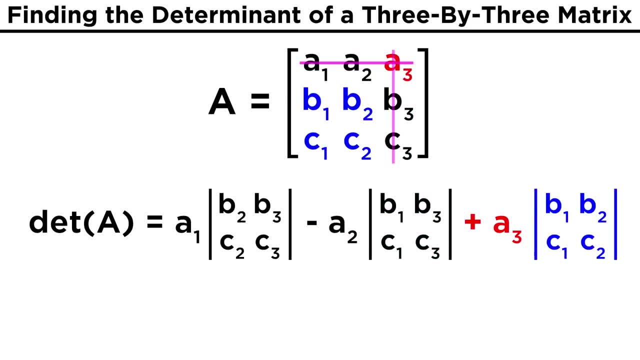 B three, C one, C three, And to that we add A three times the determinant of one more two by two matrix containing B one, B two, C one, C two. Pay close attention to the fact that we used a minus sign here and then a plus sign here. 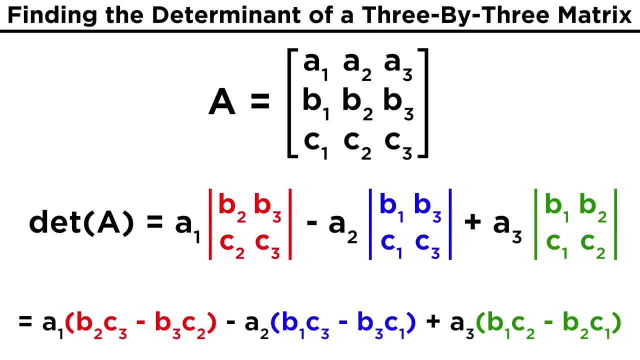 as this rule must be followed From here, we just evaluate these three simple determinants using the method we already know for two by two matrices. That would give us some products to evaluate, and we simplify until we have a final scalar value. Let's practice this with an example. 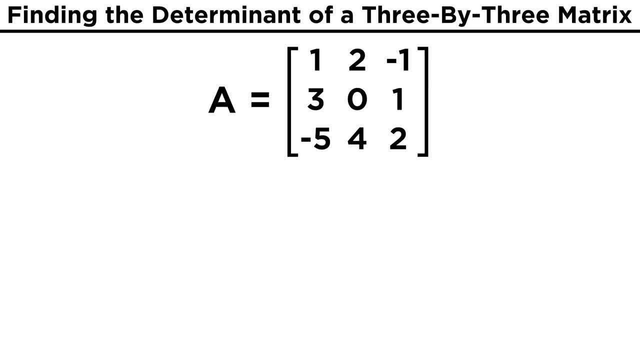 Here we see the entries: one, two negative, one, three zero, one negative, five, four, two. If we want to find the determinant of this three by two matrix, we need to find the determinant of this three by two matrix. 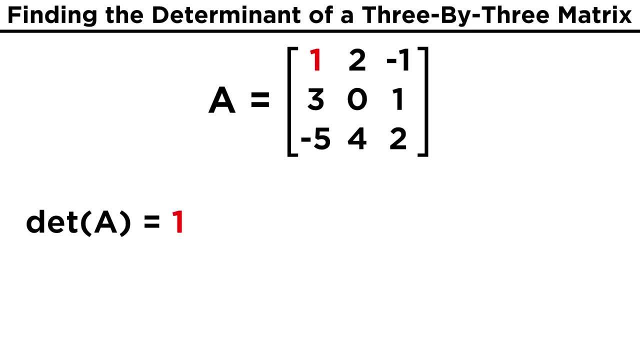 Once again, all we do is take this first entry, one, and multiply by the determinant of this two by two matrix. From that we subtract the product of the second entry from the first row two, and the determinant of this two by two matrix. 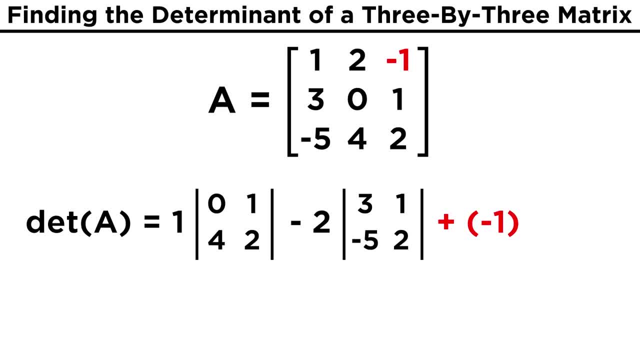 And to that we add the product of the third entry from the first row, negative one and the determinant of this last two by two matrix. Now we just have three simple determinants to calculate. The first is zero times two minus one times four or negative four. 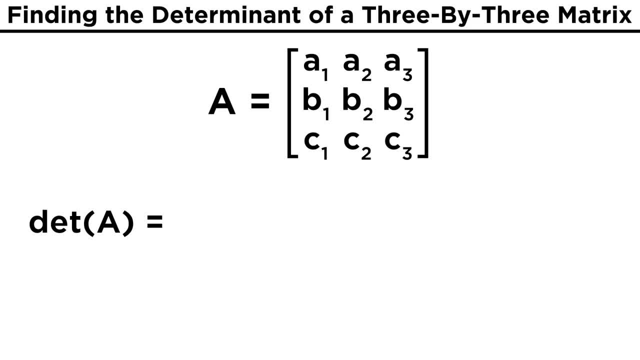 The determinant must be broken down into a series of second order determinants. We will take A one and multiply it by the determinant of a new two by two matrix comprised of B two, B three, C two, and C three. So it's like we ignored the row and column that A one is a part of, and kept the rest for a new matrix. 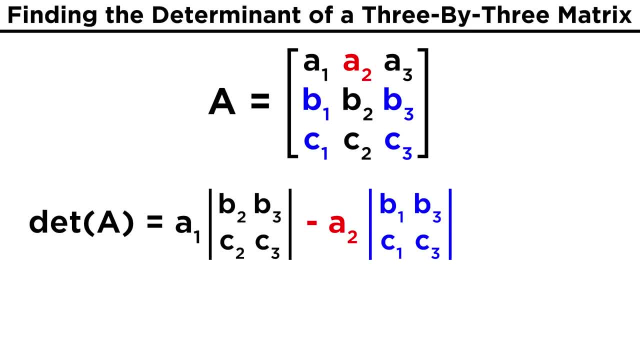 From this, we subtract A two times the determinant of another two by two matrix. This time ignoring the row and column that A two is a part of, leaving us with B one, B three, C one, C three. And to that, we add A three times the determinant of one more two by two matrix, containing B one, B two, C one, C two. Pay close attention to the fact that we used a minus sign here, and then a plus sign here, as this rule must be followed. From here, we just evaluate these three simple determinants using the method we already know for two by two matrices. 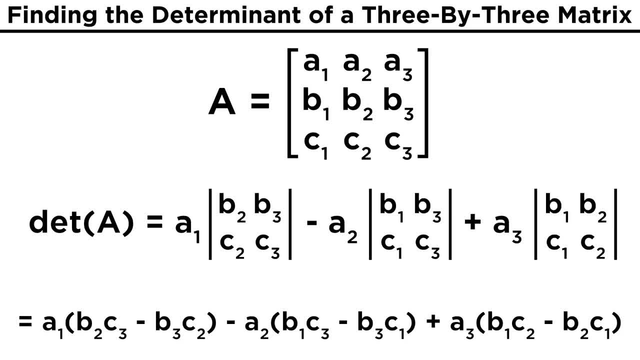 That would give us some products to evaluate, and we simplify until we have a final scalar value. Let's practice this with an example. 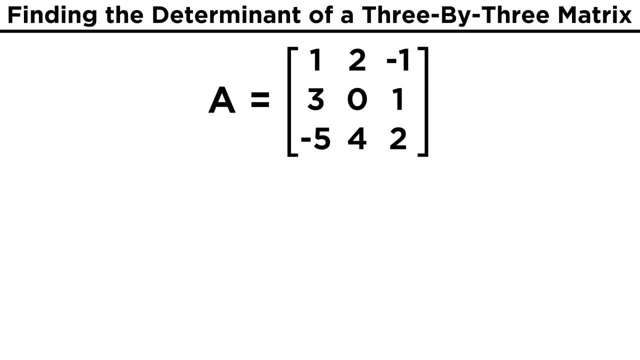 Here we see the entries one, two, negative one, three, zero, one, negative five, four, two. 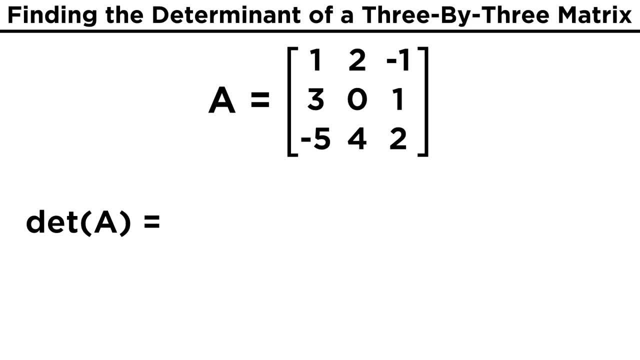 If we want to find the determinant of this three by three matrix, once again, all we do is take this first entry, one, and multiply by the determinant of this two by two matrix. From that, we subtract the product of the second entry from the first row, two, and the determinant of this two by two matrix. 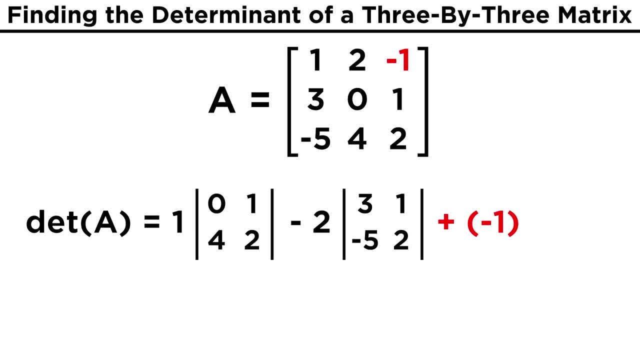 And to that, we add the product of the third entry from the first row, negative one, and the determinant of this last two by two. 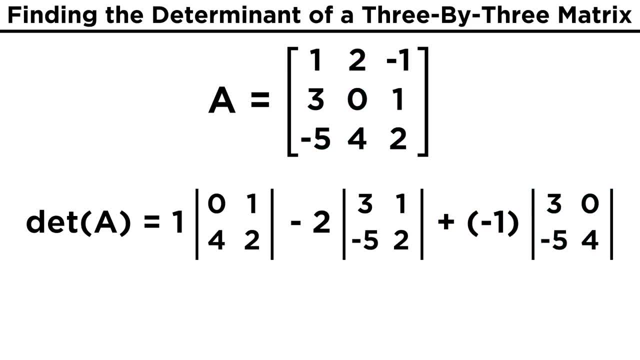 Now, we just have three simple determinants to calculate. The first is zero times two, minus one times four, or negative four. The second is three times two, minus one times negative five, or eleven. And the third is three times four, minus zero times negative five, or twelve. We multiply each determinant by the adjacent constant. Then, we multiply by the adjacent constant. 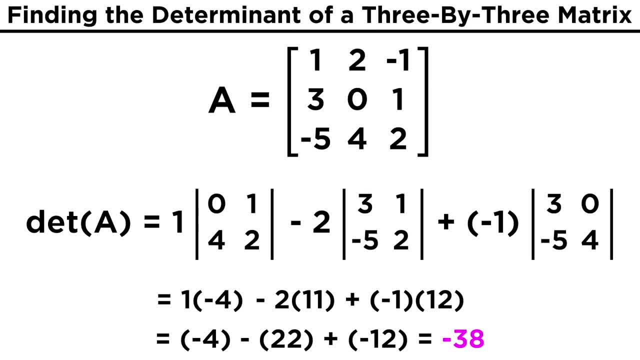 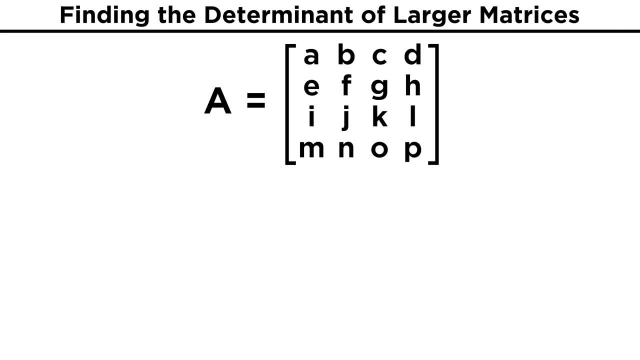 We perform the addition and subtraction, and we should get negative thirty-eight as our answer. 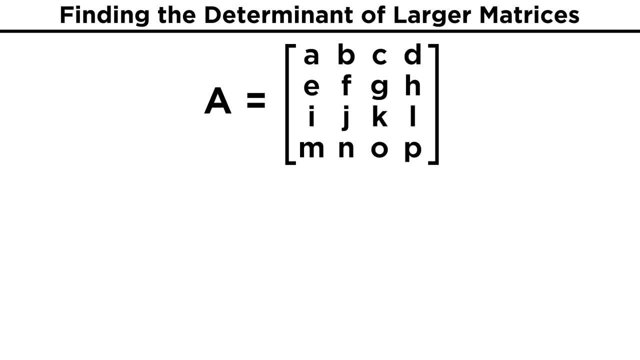 Now how would we find the determinant of larger matrices still? As the matrices get bigger, the algorithm doesn't really get any harder, we just end 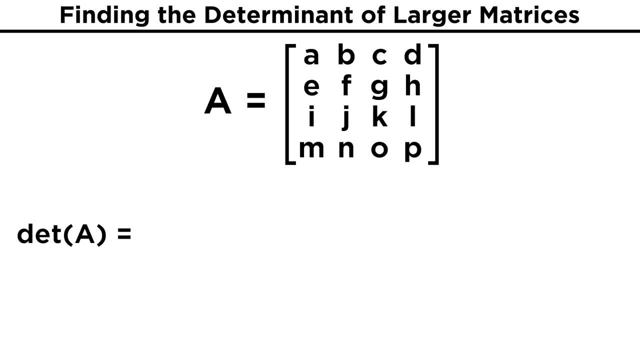 up adding many more steps very quickly. For a four by four matrix, we will take the first entry, and multiply by the determinant of this three by three matrix. Minus this second entry times the determinant of this three by three matrix, plus the third entry times the determinant of this three by three matrix, minus this fourth entry times the determinant of this three by three matrix. 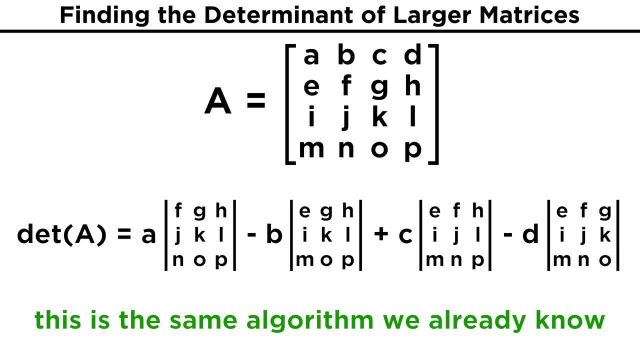 So we are doing the same thing we did before, going across the first row and blocking out the row and column containing a particular entry, and multiplying by the relevant determinant. But what if I take all my entries and subtract them, and the Poisson formula is nothing but an integral from this column? 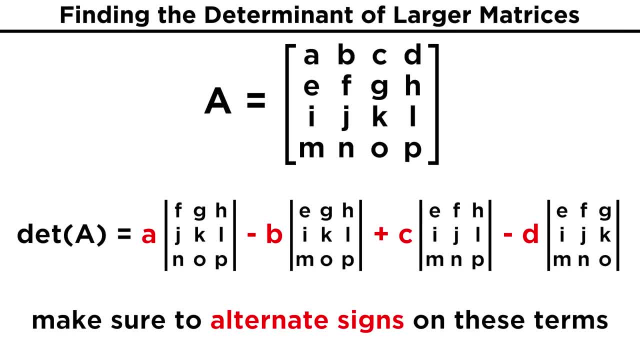 Also, notice that we subtract a term, then add the next, then subtract the next. This would continue alternating for as many terms as were necessary. 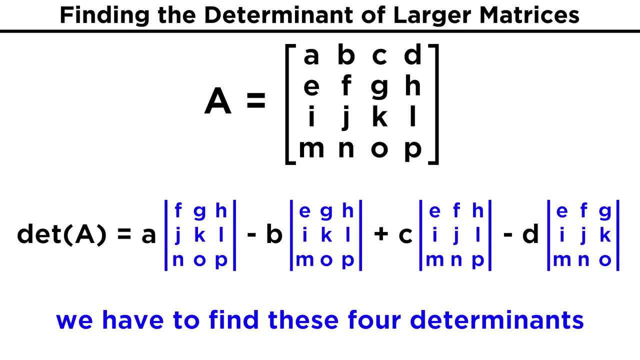 Now that we are here, we have four separate three by three matrices that we need to find determinants for, and as we just learned, each of these will involve the determinants of three separate two by two matrices. So we have definitely made quite a bit of work for ourselves, but as long as you remain organized and stay on top of your arithmetic, there is no reason that you can't find determinants for matrices of this size or even larger. 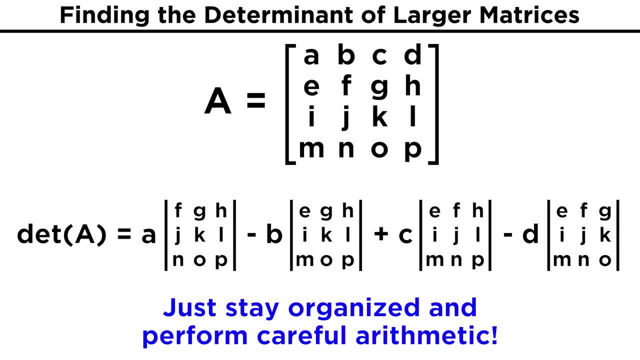 Now that we know how to find the determinant of a matrix, let's check comprehension. 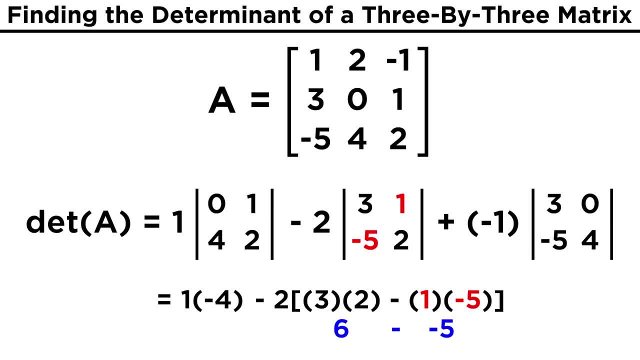 The second is three times two minus one times negative five or eleven. And the third is three times four minus zero times negative five or twelve. We multiply each determinant by the adjacent constant, then we perform the addition and subtraction And we should get negative thirty-eight as our answer. 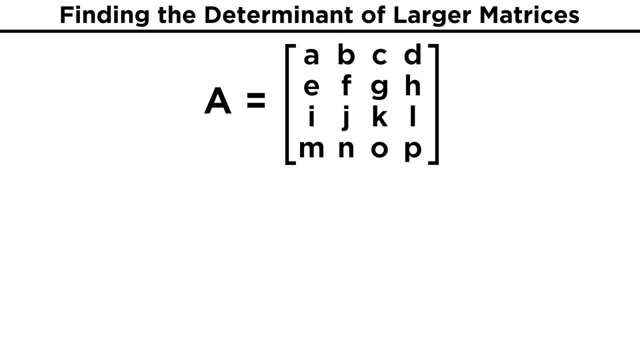 Now how would we find the determinant of larger matrices? still, As the matrices get bigger, the algorithm doesn't really get any harder. we just end up adding many more steps very quickly. For a four by four matrix, we will take the first entry and multiply by the determinant. 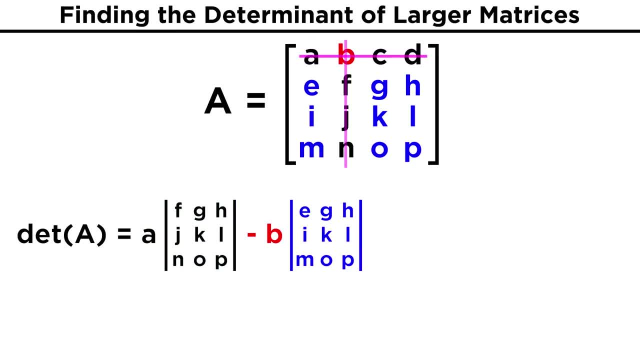 of this three by three matrix Minus one by two Minus this second entry times the determinant of this three by three matrix Plus this third entry times the determinant of this three by three matrix Minus this fourth entry times the determinant of this three by three matrix. 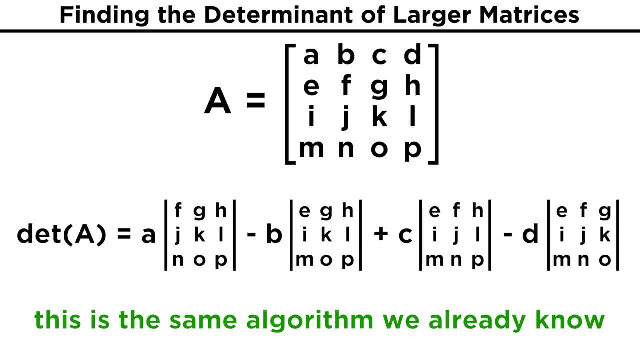 So we are doing the same thing we did before, going across the first row and blocking out the row and column containing a particular entry and multiplying by the relevant determinant. Also, notice that we subtracted- Subtract a term, then add the next, then subtract the next. 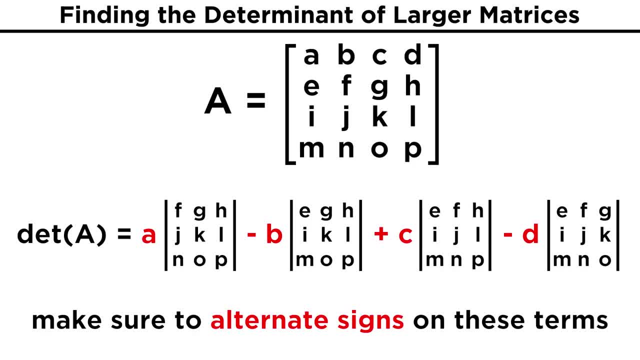 This would continue alternating for as many terms as were necessary. Now that we are here, we have four separate three by three matrices that we need to find determinants for and, as we just learned, each of these will involve the determinants of three separate two by two matrices. 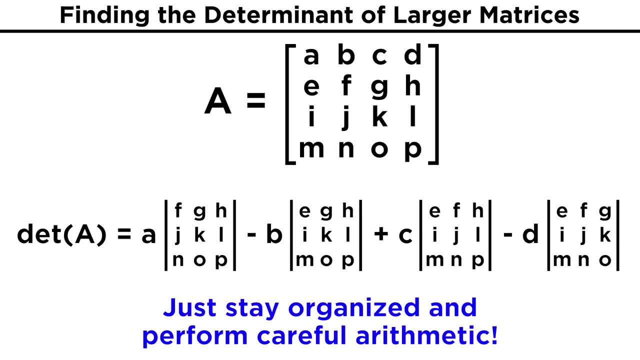 So we have definitely made quite a bit of work for ourselves. but as long as you remain organized and stay on top of your own matrix, you will be able to find determinants for your own matrices. Even if you don't know your arithmetic, there is no reason that you can't find determinants. 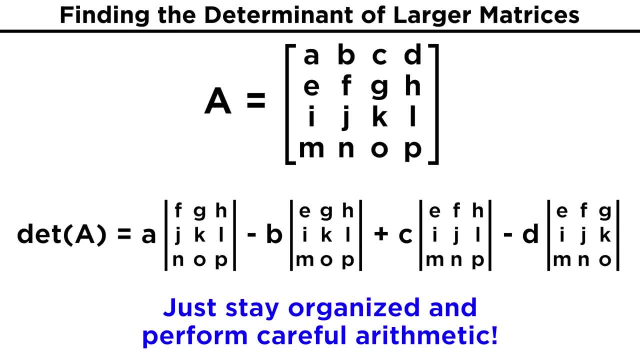 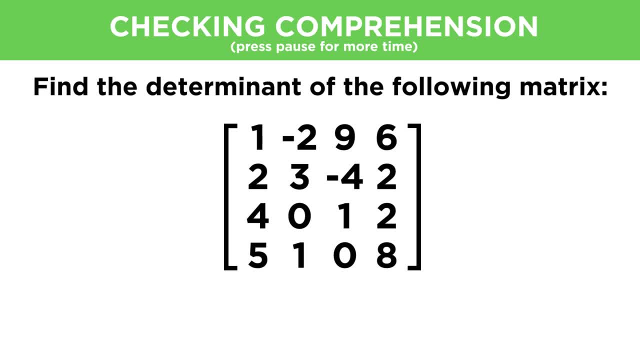 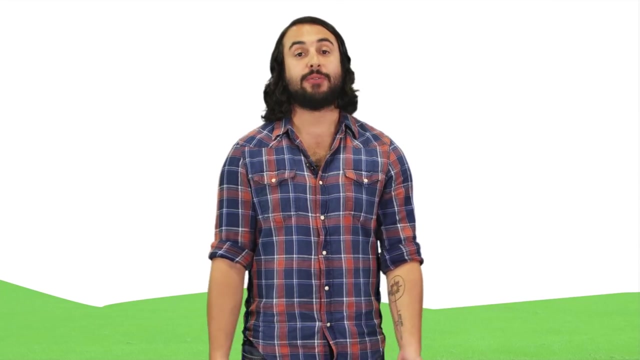 for matrices of this size or even larger. Now that we know how to find the determinant of a matrix, let's check comprehension. Thanks for watching, guys. Subscribe to my channel for more tutorials. support me on patreon so I can keep making.